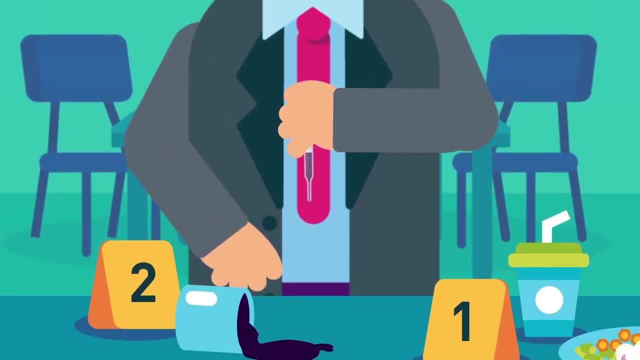 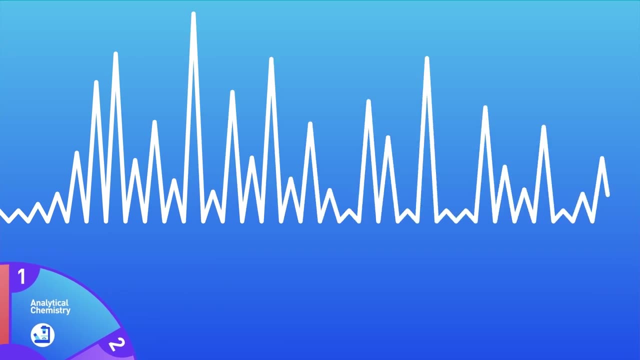 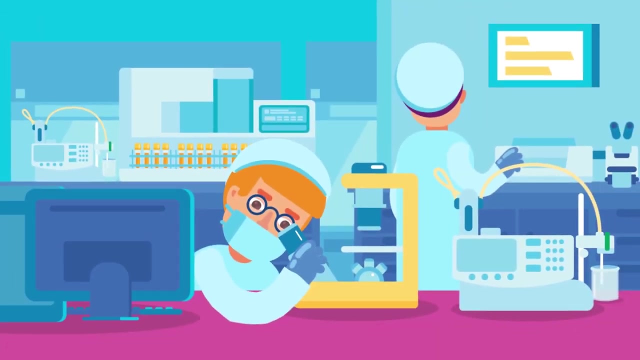 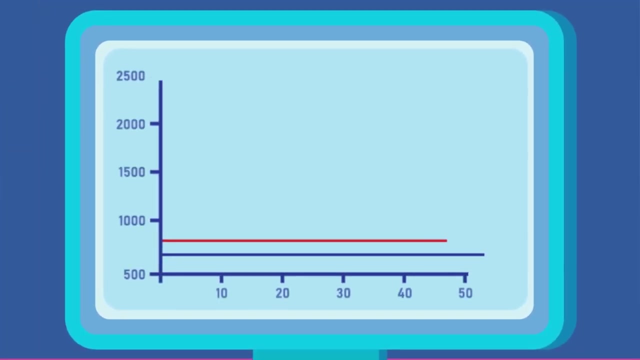 using analytical chemistry include forensic science, environmental science and drug testing, Analytical chemistry. Analytical chemistry can be divided into two main branches: Qualitative and quantitative analysis. Qualitative analysis employs methods and measurements to help determine the components of substances. Quantitative analysis, on the other hand, helps to identify how much of each 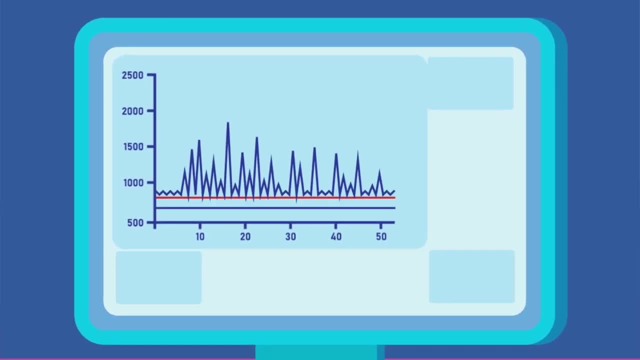 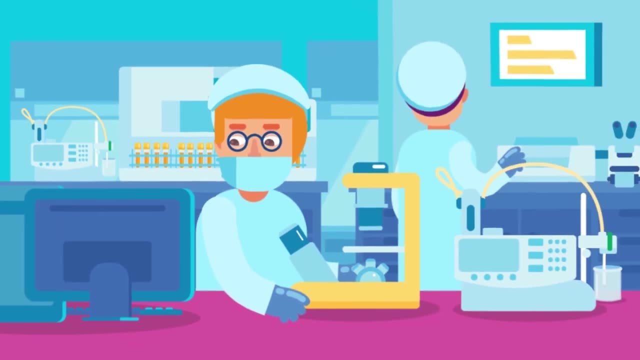 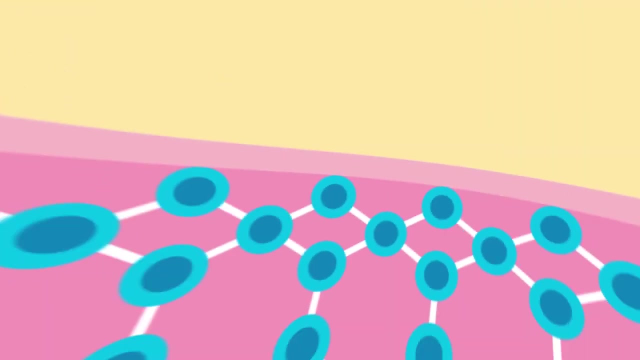 component is present in a substance. Both types of analysis can be used to provide important information about an unidentified sample and help to identify what the sample is. reinforces that a NEED is. ocean suppliers are looking for sobre to detect whether or not a restricted sample is present. More information about both methods requires accurate analysis. 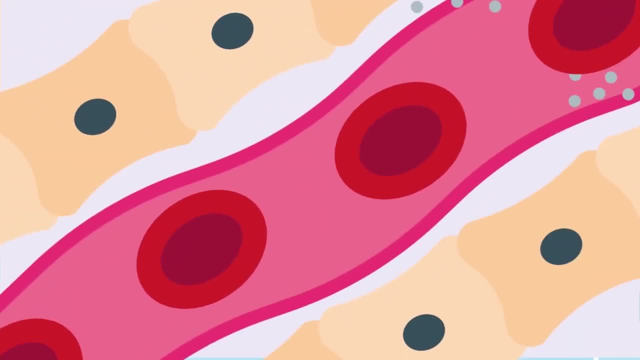 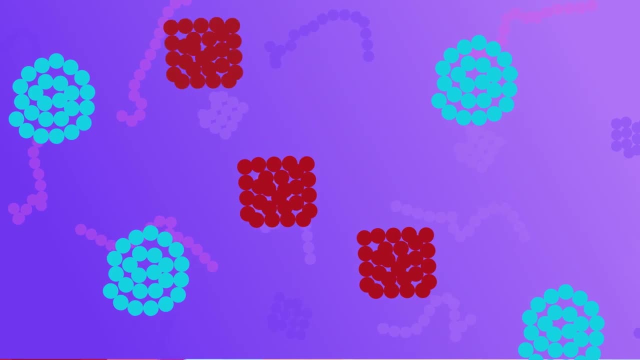 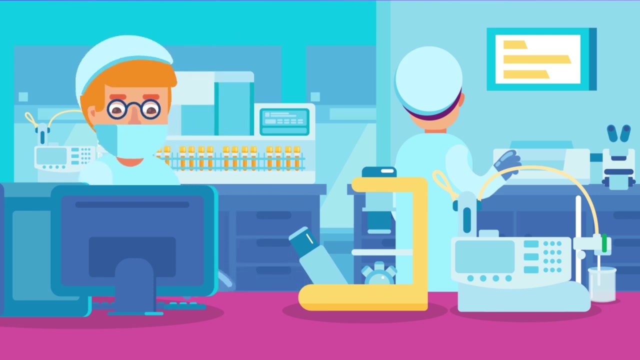 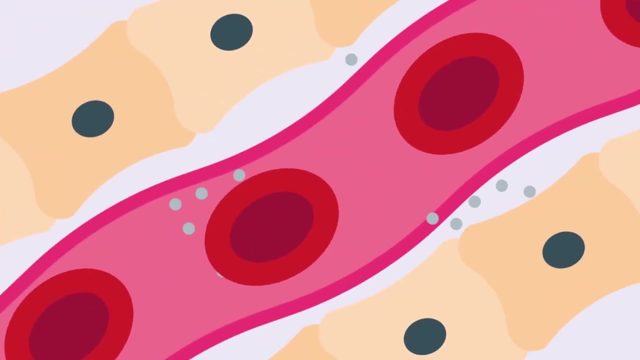 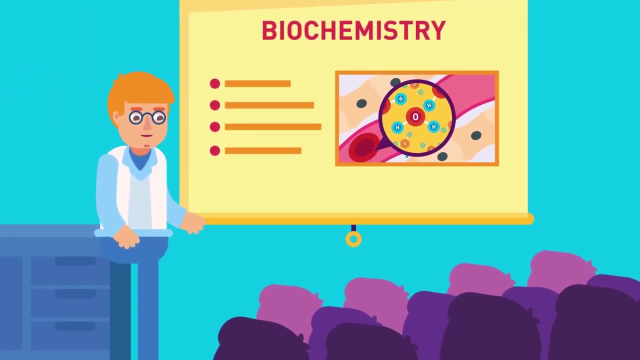 Perspectives against biological processes: Implementation. explaining Biochemistry: Symptoms A Four school number hundred. take Learn more at. Everything in the body is made up of atoms and molecules, of different chemical compounds like carbon, oxygen and hydrogen. This is what we study in biochemistry. 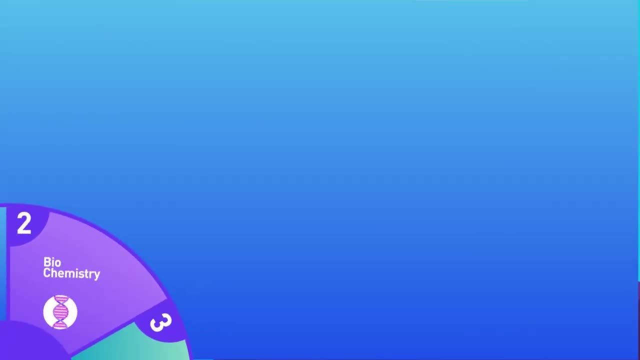 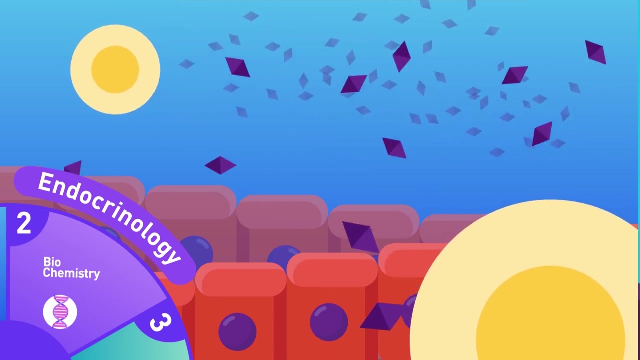 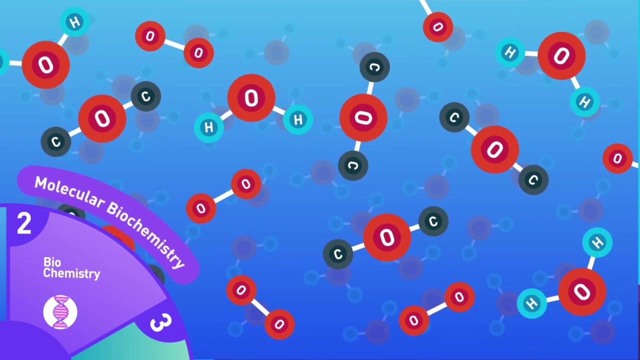 Biochemistry can further be divided into interesting disciplines like Enzymology, which is the study of enzymes, Endocrinology, which is the study of hormones, Clinical Biochemistry, which is the study of diseases. Molecular Biochemistry, which is the study of biomolecules and their functions. 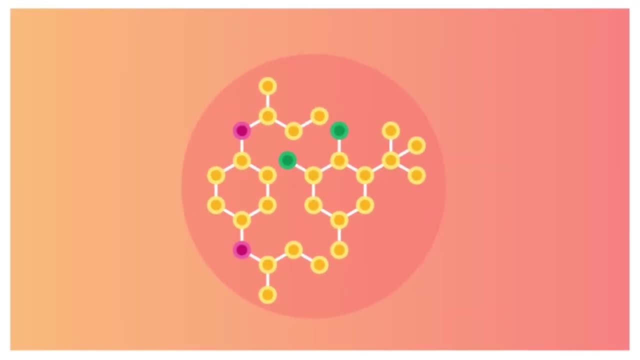 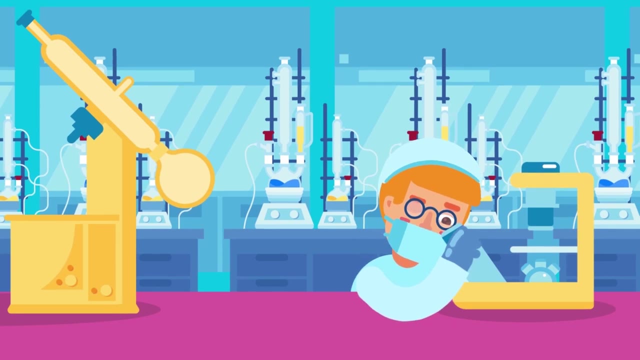 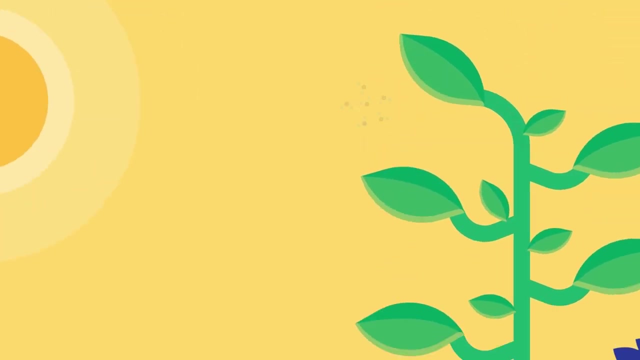 Organic Chemistry: the study of carbon compounds such as fuels, plastics, food additives and drugs. Organic Chemistry deals with the study of carbon and the chemicals in living organisms. An example is the process of photosynthesis in a leaf. because there is a change in the 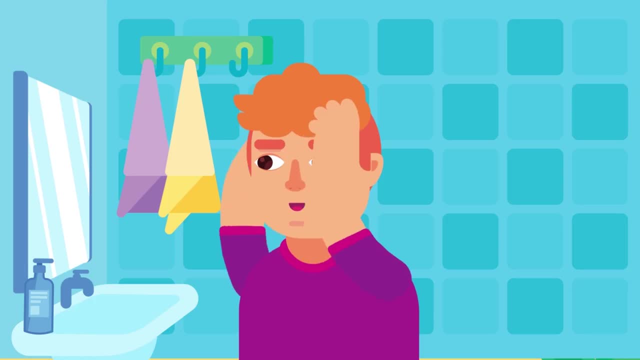 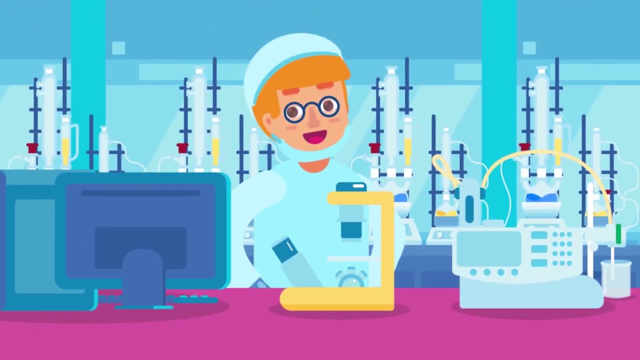 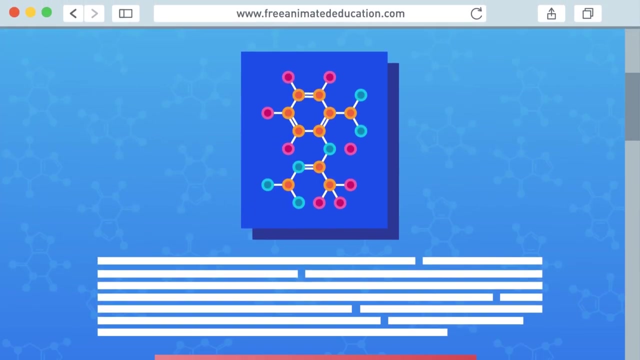 chemical composition of the living plant. Have you ever wondered who makes your hair? Have you ever wondered who makes your hair? Organic Chemists are the ones who do these. They devise experimental methods to isolate or synthesise new materials and study their properties.